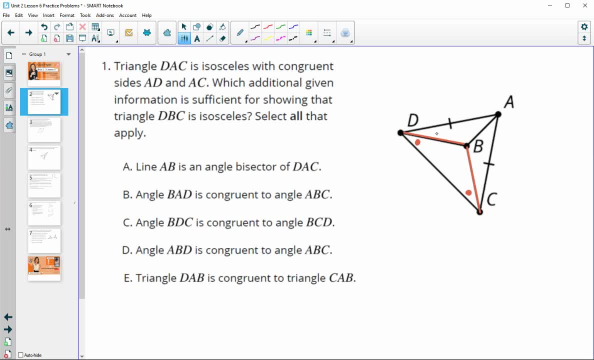 And then when we know that the base angles are congruent, that would prove that it's an isosceles triangle as well. So those are the two things we're kind of looking for with the information that they're giving us. So A says if line AB. 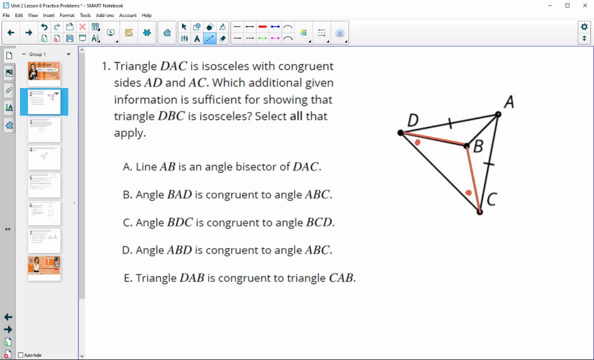 is an angle bisector of DAC, would that be enough to prove that that's isosceles? So not directly, but it actually does work, because if this is the angle bisector, then that means that this angle is congruent to this angle, And then we know that AB is the. 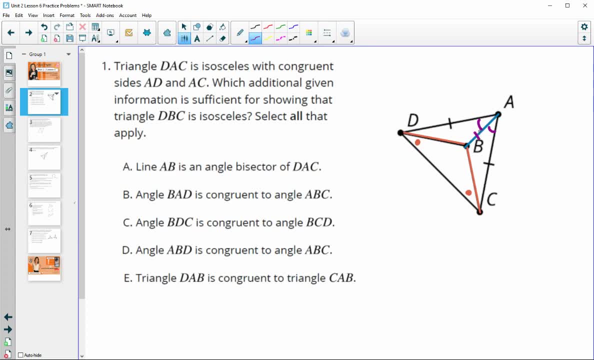 same segment in both triangles. So we know that this is congruent. So then we actually have in each triangle, this side, this angle and this side congruent. So we have side angle, side to prove that these two triangles are congruent, which then we know, ultimately tells us that this 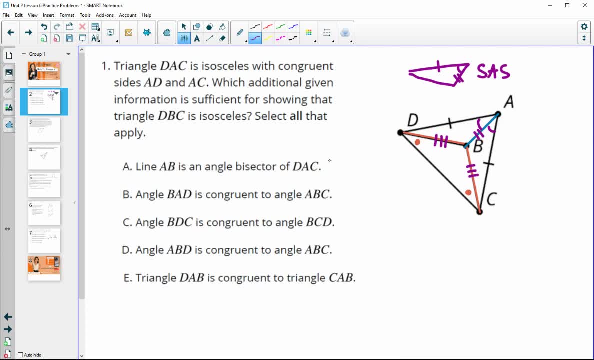 side is congruent to this side because of corresponding parts, because they would be corresponding parts of these two congruent triangles. So this one will be true And I'm just going to make a little note here that we proved that DB. well, let's put, I'm just going to say, because this forces the triangles to be congruent by side. 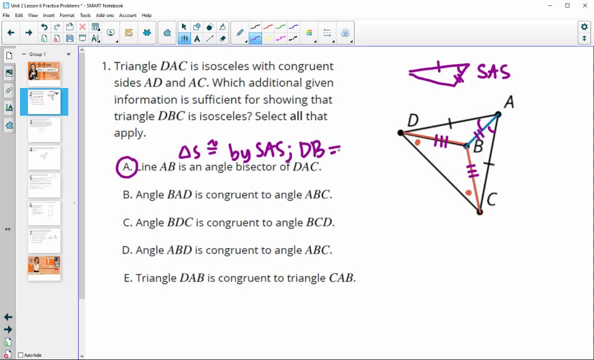 angle side and then DB would be congruent to BC because they're corresponding parts of those congruent triangles. All right, then let's clear this out. All right. next one asks us or tells us what if we knew that angle BAD, so this angle here? oops, let me use a. 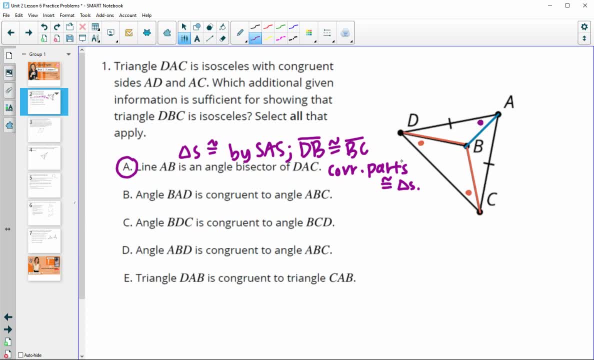 different color, that this angle here was congruent to ABC, so this angle. So would it help us if we knew that those two angles are congruent? And no, that wouldn't help us prove the triangles are congruent or get these base angles. So this one doesn't help. Angle DBC, so DBC. 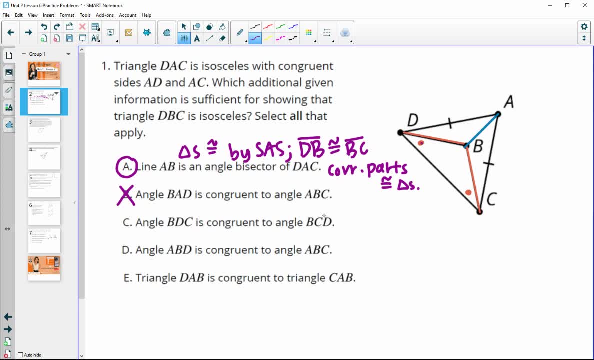 is this one congruent to BCD? this one. So we know that would help because that would tell us that we have congruent base angles. So then we would know it's isosceles by that base angle, theorem Angle ABD. so ABD is this one? congruent to ABC? would be this one. So we still have that same. 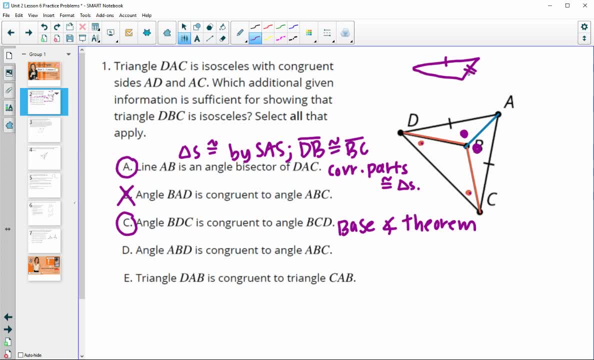 segment, but we still have that same segment, but we still have that same segment, but we still have segment in both. So now in the triangles we would have this And that doesn't help us because it's not the included angle, So that won't help us prove that those two triangles are congruent, So that 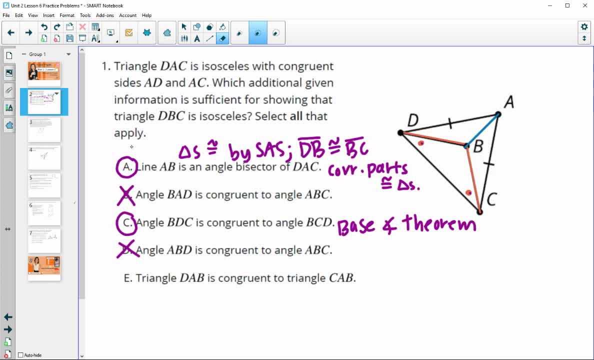 information is not useful to us for this task. Then triangle D. if they just told us triangle DAB, so this triangle was congruent to CAB, if they just tell us straight up that those triangles are congruent, that would be helpful. 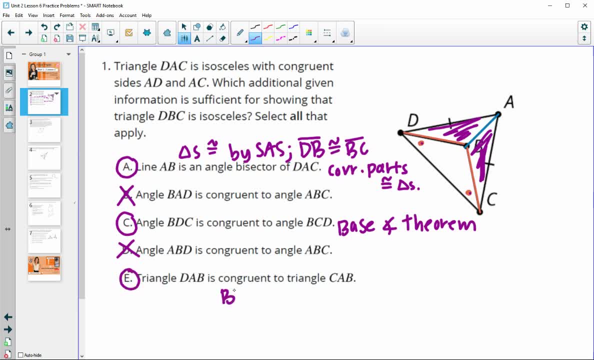 Because then we would know that BD is congruent to BC again, because they are corresponding parts of those congruent triangles. So then that would make this side be congruent to this side, which by definition makes that an isosceles triangle. 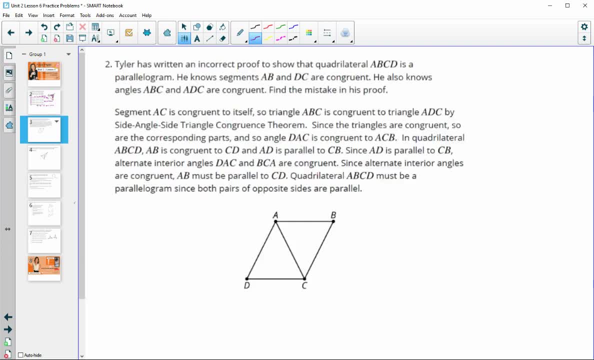 All right. number two says that Tyler's written an incorrect proof. So he's written an incorrect proof to show that this quadrilateral is a parallelogram. The things that he knows are that segments AB and DC are congruent, And he also knows that angles ABC and ADC are congruent. 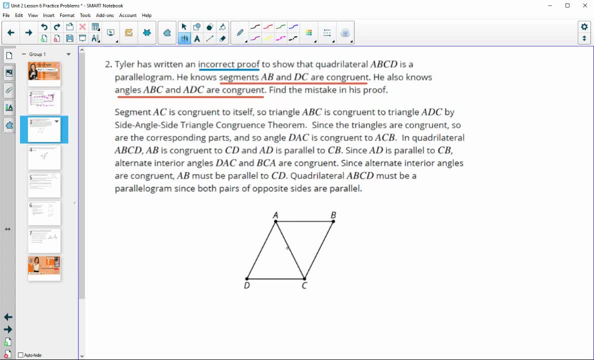 So I'm going to mark that on here first. So he knows that AB and DC are congruent And he also knows that angle ABC, which is this one, is congruent, And he also knows that angle ADC is congruent to ADC, which is this one. 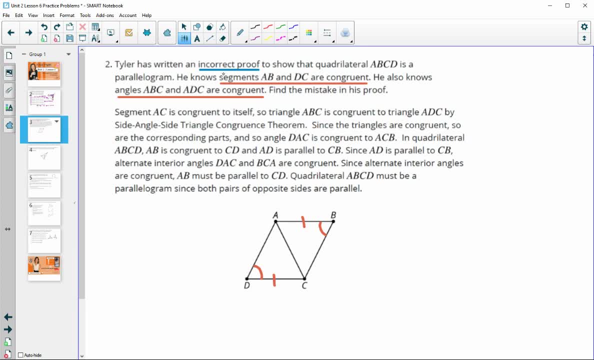 So he starts off as proof by saying: segment AC is congruent to itself, which is true, So he has this in there. Then he says: so triangle ABC is congruent to ADC by side-angle-side congruence theorem, And that's where he goes wrong. So side-angle-side congruence theorem. 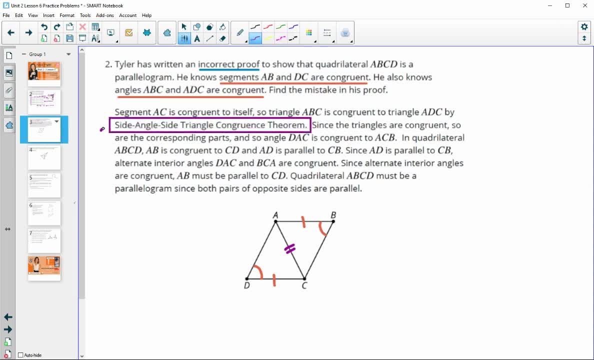 this is not true. Okay, so this is false because he doesn't have the included angle. The included angle would be here. He doesn't have that, Okay, so false. He does not have two sides with an included angle, So side-angle-side- whoops- does not work. 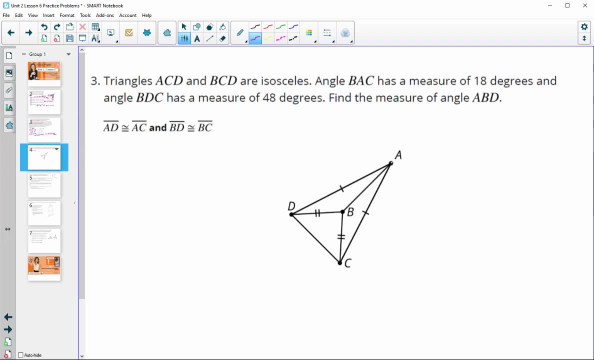 All right. number three says that triangle ACD, so this big triangle here is isosceles and BCD. this littler triangle is isosceles, Angle, BAC, so this one here is 18 degrees, Find sorry. and BDC, so this one here is 48 degrees. 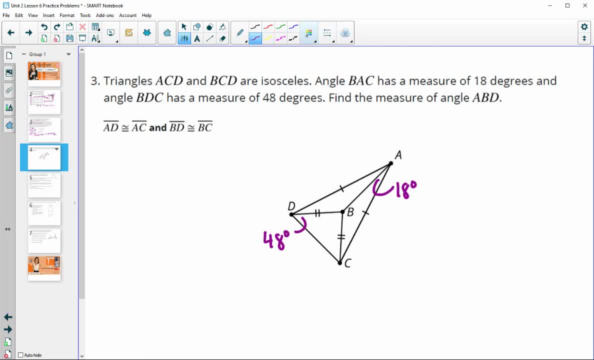 Find the measure of angle ABD. So we want to find the measure of ABD, which is this angle here. So we're looking for this one. So we see kind of this segment A. well, we can look at segment AB here as being congruent to ABD. 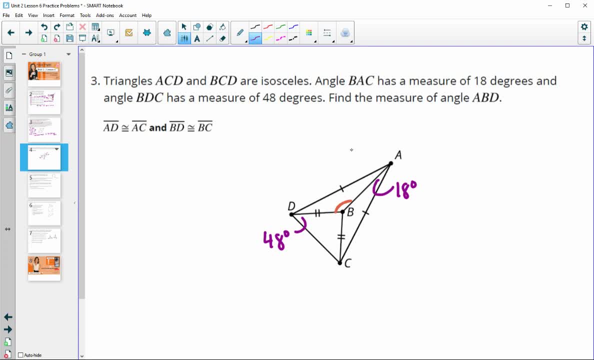 So we know that these two triangles are equal. So we do know this angle here which maybe could be helpful. So we know this one is also 18 degrees. Isosceles triangles would say that this big angle here is congruent to this big angle here. 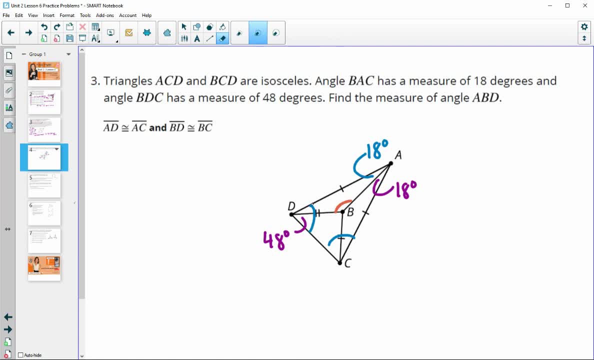 And we don't know these kind of little top angles, So that's not really helping us right now. But what we also know is this little isosceles triangle here. this would be a base angle with this. so we know that this one is 48 degrees because it's a base angle, and then that'll. 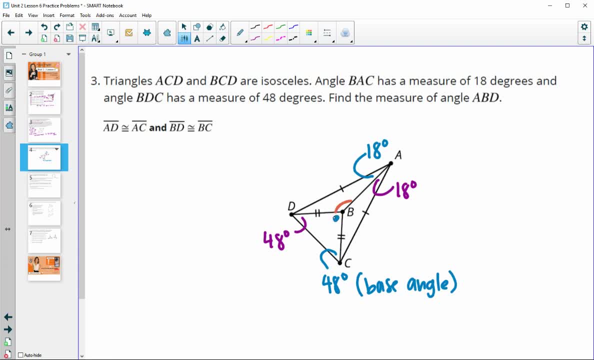 actually help us find this angle here. so there's kind of two ways. so this is one way. so we could find this angle here by doing 180 minus 48 minus 48 and that's gonna give us 84 degrees here for this angle and the reason that that one could. 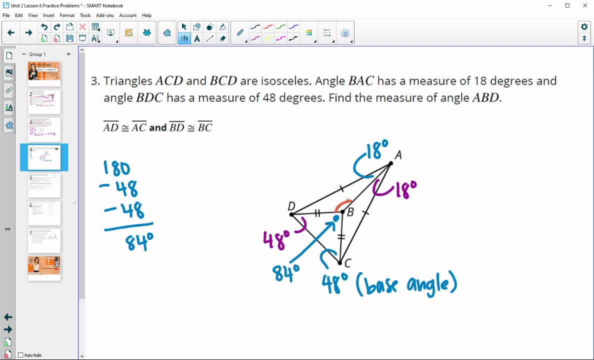 be helpful to us is that we know that these two angles are equal in size, and if you look at this, you could see that this whole thing makes a circle, and so we know that a circle is 360 degrees, so we could do 360 minus the 84, which gives us 276 degrees left over for these. 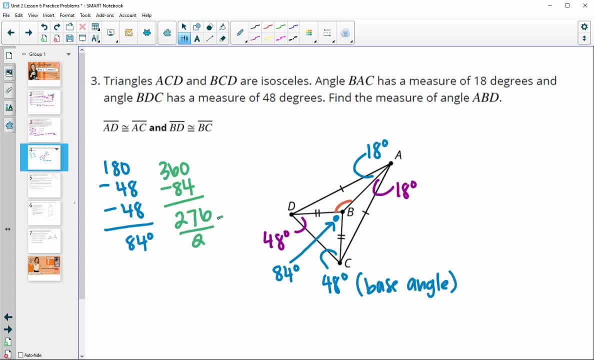 two angles, and so then we could divide that by 2 and that would give us 138 degrees there, and that would be the measure of angle ABD. so 138. so that's one way to get to it. another way that you could get to this would be by 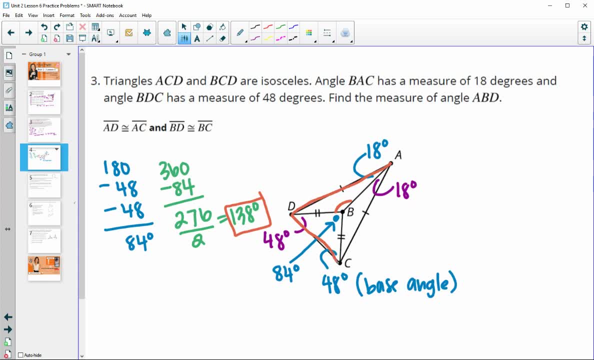 looking at this bigger isosceles triangle, and so you know that that totals 180 degrees. so we could do 180 minus these two 18s for this angle here. so two 18s is 36, and that would give us 1044 degrees, in which case we could divide. 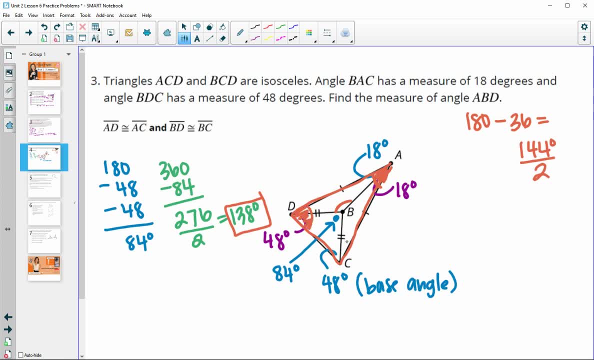 that by 2 to get these kind of bigger base angles here, because we know these are the same and so that's gonna equal 64 by 3 and 72 degrees. So that would help us to find one of these kind of little angles here. So we know this. 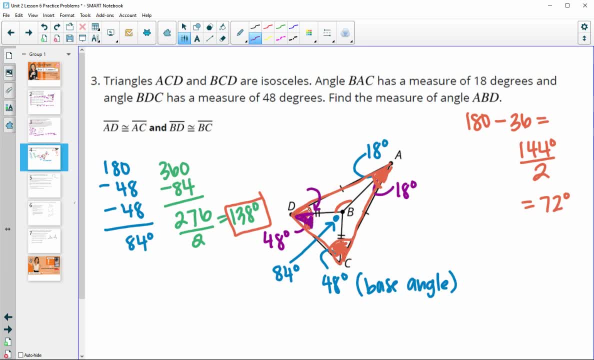 piece was 48. Okay, now it would help us find this other angle here, So we could subtract 48 from here and get what is that 24.? So then we'd get 24 degrees here And then we could subtract these. 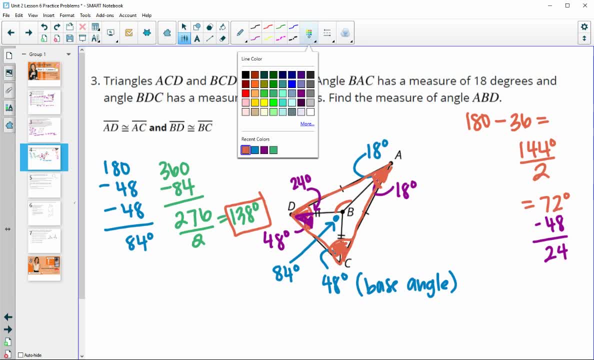 two from 180 to get that whole triangle. So to figure out this other angle here, we could do 180 minus 18, which is 162, and then minus the 24,, which would give us 138 degrees again. So two kind of different ways, depending on how you see it. 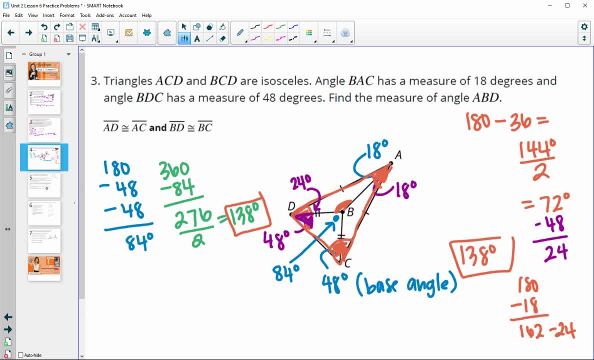 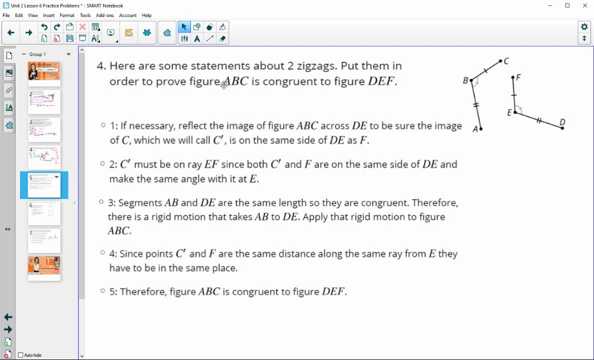 One is probably going to feel more comfortable than the other. All right, number four: here's some statements about two zigzags. Put them in order to prove that figure ABC is congruent to figure DEF. So when I'm looking at this, instead of getting 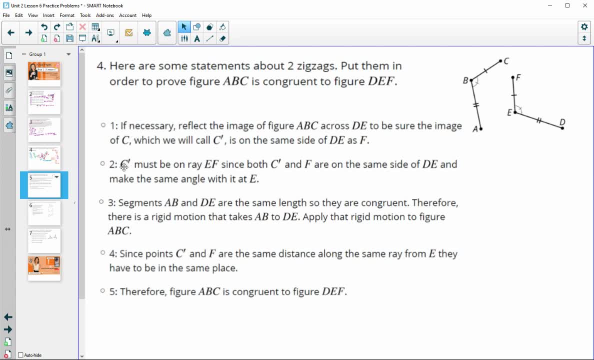 lost in all of the words right away. I kind of look at the starting parts of the sentences to see if that tells me anything and if that'll help me kind of narrow my choices down. So this one says if necessary, which tells me it's probably not the first one. So I'm going to look at the 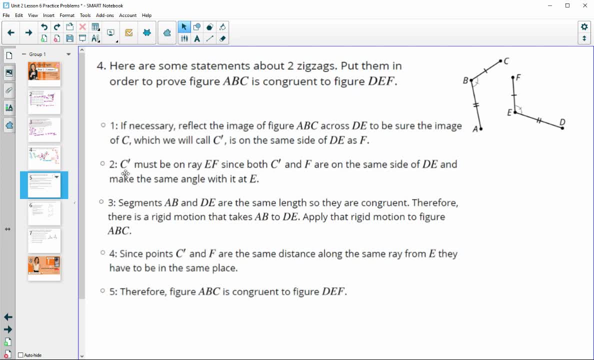 statement. So something else probably happened first. Number two starts with C prime, which is an image, meaning something has happened already. So that's probably not first. This one just starts talking about segments that are the same length, So that has a possibility of being first. 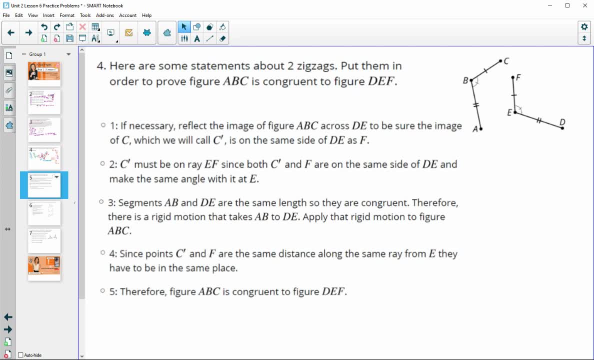 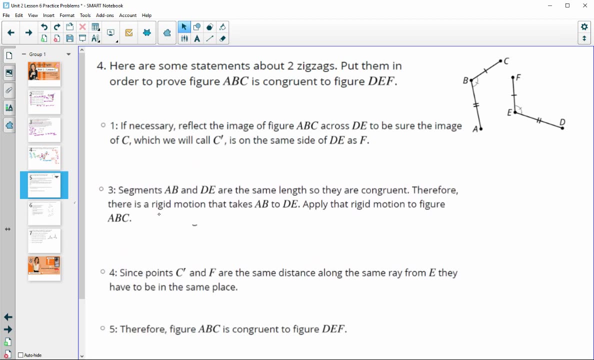 Number four has the word since in it, So again, not going to be first, And then number five says therefore. So the word therefore tells me that this is my last statement, And then kind of what I narrowed it down to is: this is probably my first statement, So I'm just 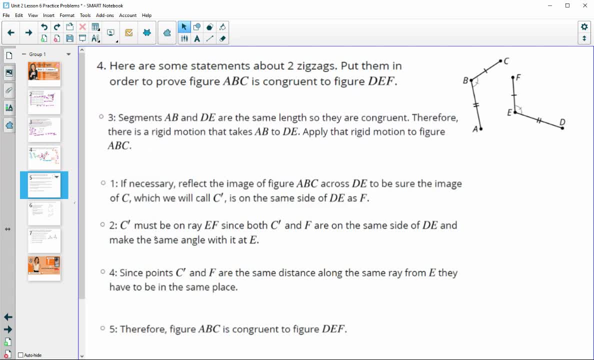 going to pull that up to the top and read it and make sure it could be the first statement now. So segments A, B and D are congruent. Okay, A, B and D are congruent, So they're the same. 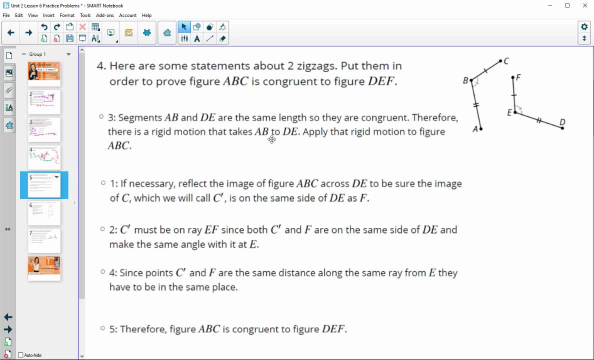 or sorry. they're the same length, So they're congruent. Therefore, rigid motion takes A, B to D. E apply that rigid motion, So this one just had us move this zigzag onto this one, So we know this segment is. 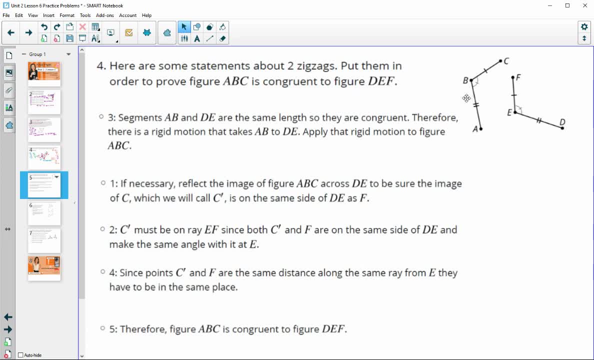 congruent to this one. So we just translated it, or did the rigid motion? a translation and a rotation. So this is our first statement Now that we've gotten this kind of zigzag on here. if you remember, there's a potential to. 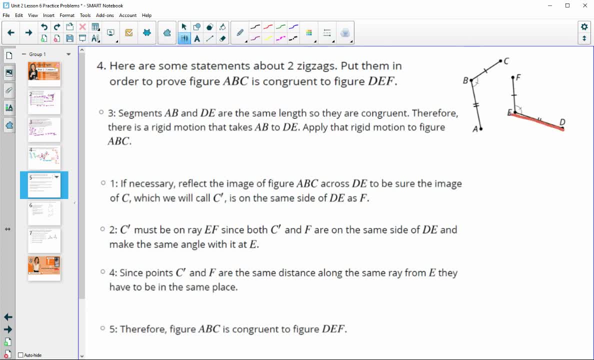 need to reflect it, in case this zigzag was actually this way. So that's where this if necessary part comes in, So we get those segments on top of each other. Then, if it's necessary reflect it In this case, we're going to reflect it. So we're going to reflect it. So we're going to. 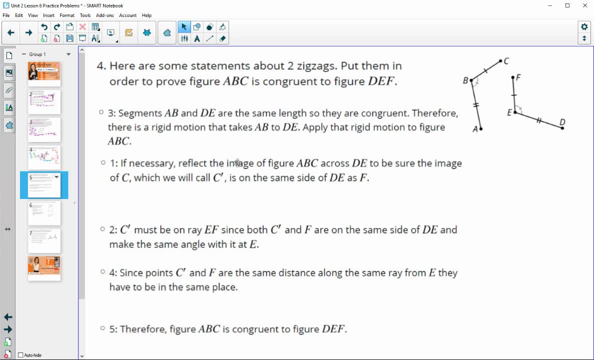 reflect it. In this case we're going to reflect it. So we're going to reflect it. So we're going to reflect it. In this case it's not necessary, But if necessary we would reflect it. And so then now it's saying: so now we're kind of looking between these two. So then it says: 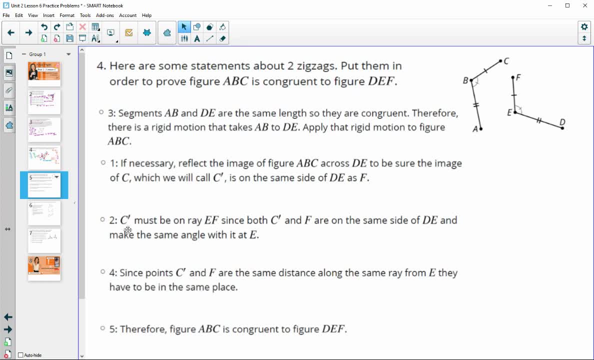 sense points C and F are the same distance along the ray, or C prime must be on ray EF. So this one here says that we already know that they're on the same ray. This one here is saying it must be on ray EF. So this statement is proving it to us that they're on the same ray. 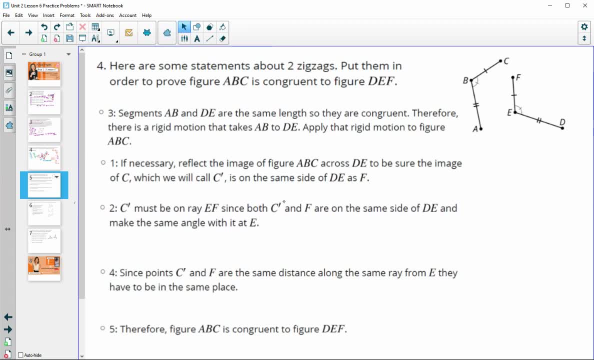 So C- prime must be on ray EF, since C, prime and F are on the same side of DE. And then this one tells us: since C and F are the same distance along the ray, then they have to be in the same place And then, ultimately, therefore, the figures are congruent. 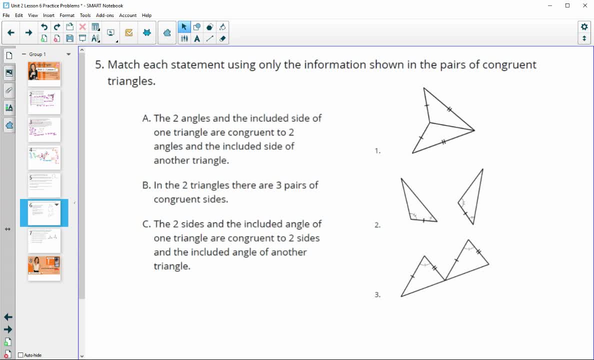 Number five match the information with the diagrams. So part A says that we have two angles and an included side. So let's look for two angles and an included side. That's happening in number two. B says a triangle with three pairs of congruent sides. 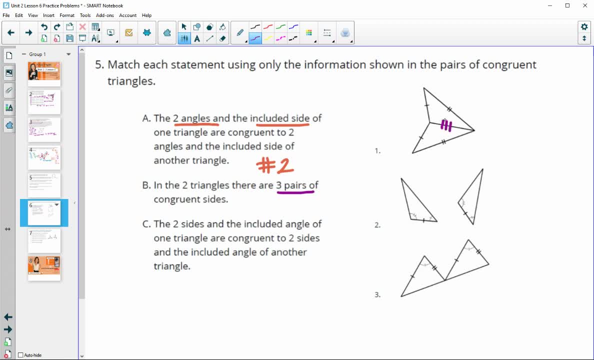 And so we see that here too. but then we also know two sides, but then we also know this one's the same in both. So that's our third. So that's number one, And then that would leave number three for part C. 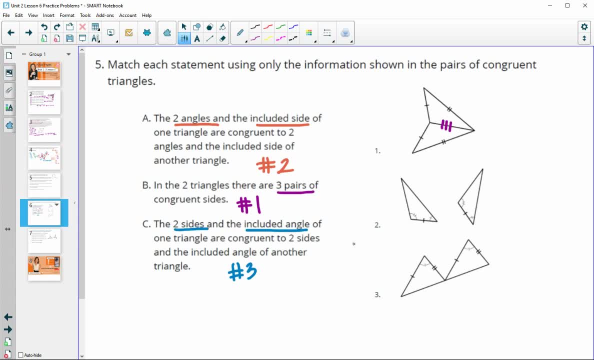 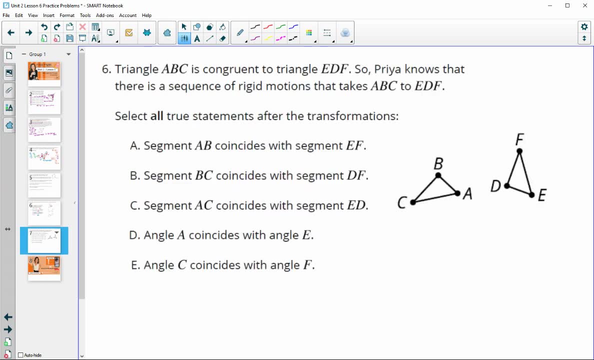 And we could just look and make sure two sides and the included angle, So two sides with that angle in between, is number three. All right. Then number six says triangle ABC is congruent to EDF. So there is a sequence of rigid motions that takes one to the next. 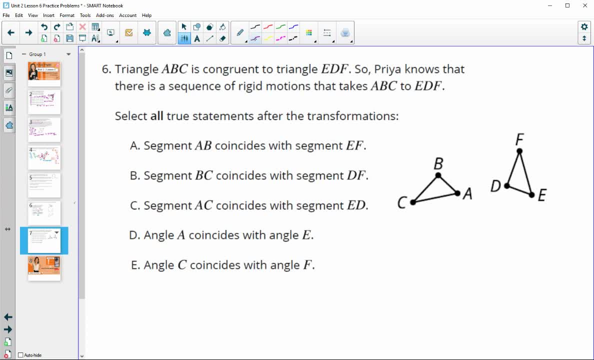 Select all true states And then we can look at the statements after the transformation has been applied. So again, you can look at the picture. These two triangles look fairly similar, So they're kind of hard to look at, in my opinion. 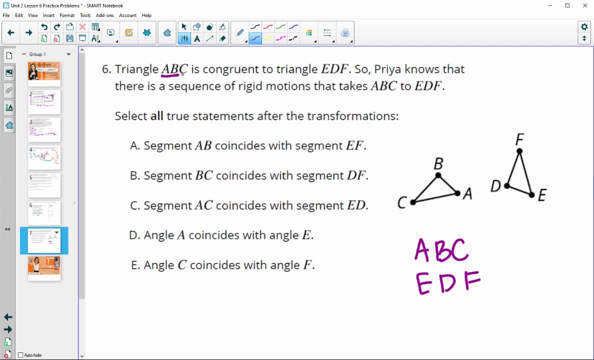 So I'm just going to write these two triangles that they gave me that are congruent, right on top of each other, So I can see the corresponding pieces And then look at it that way. So A says that AB coincides with EF. 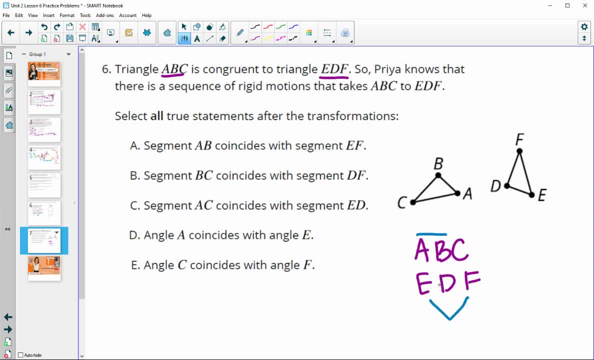 So AB coincides. Those are not matched up, So that is false. BC coincides with DF. Those are in the same spot, So those are corresponding and therefore equal. AC coincides with ED. So first and last with the first. two are not corresponding. 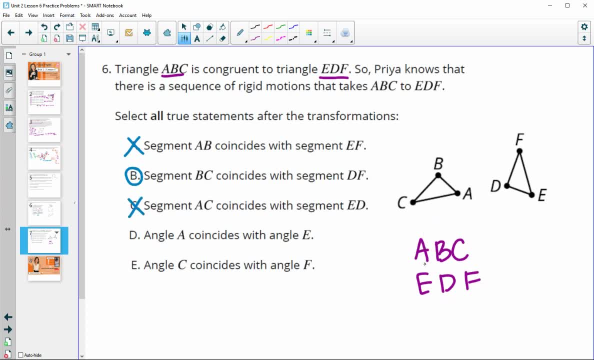 So those will not coincide. A coincides A coincides with E: Yes, C coincides with F: Yes.